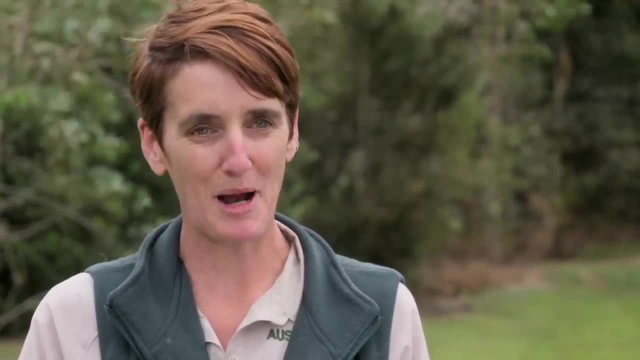 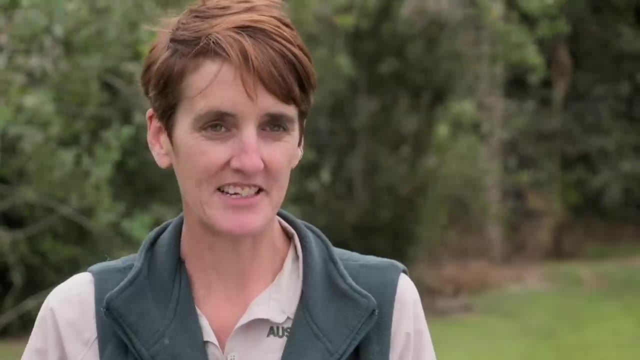 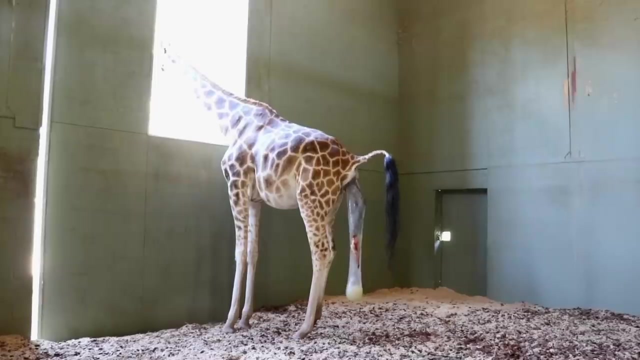 her abdomen because of that, But she's been through this before so she's pretty used to what's happening. It's all right. The stages of labour for Rosie and for any giraffe are pretty much the same as for any other animal, So first of all the water will break and then the fluid will be expelled from around the sac. 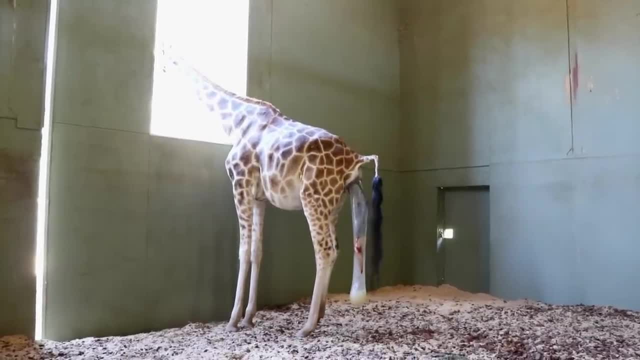 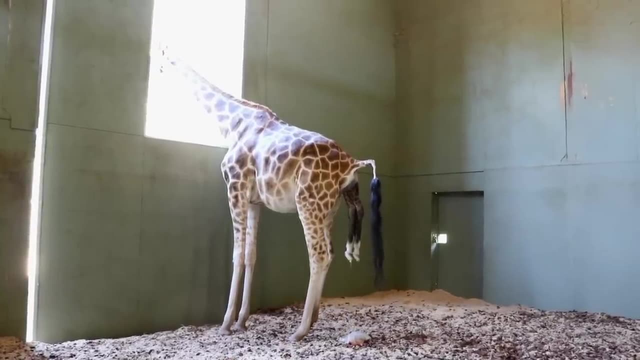 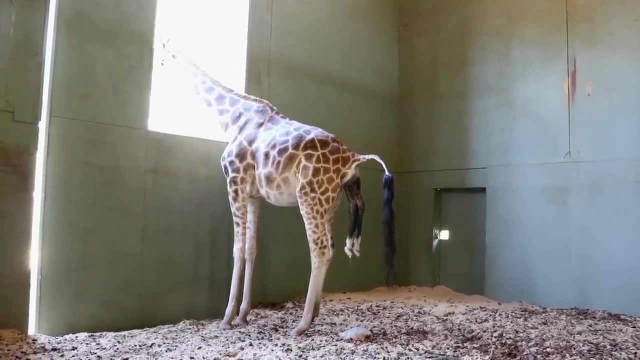 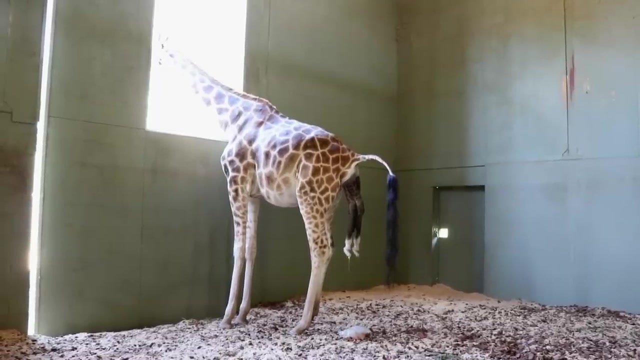 which encloses the foetus, and then the baby comes out. Good girl, Rosie, It's all right. Giraffe, birth is um pretty dramatic. The newborn falls from quite a height and hits the ground with um quite heavily, So there is a little bit of a risk of injury, but it's all up to the gods. 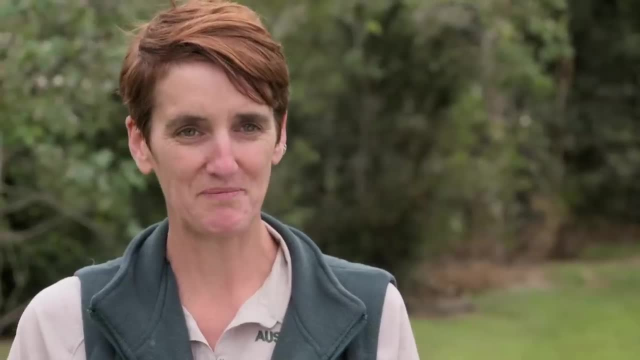 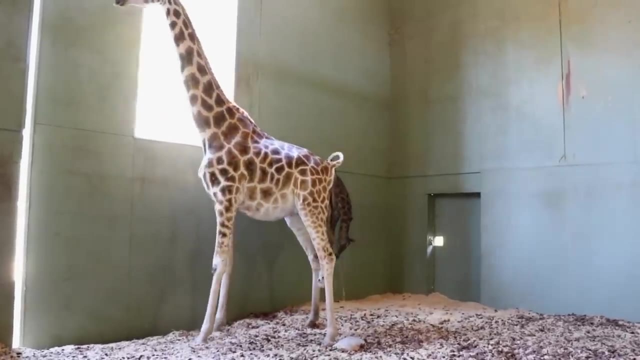 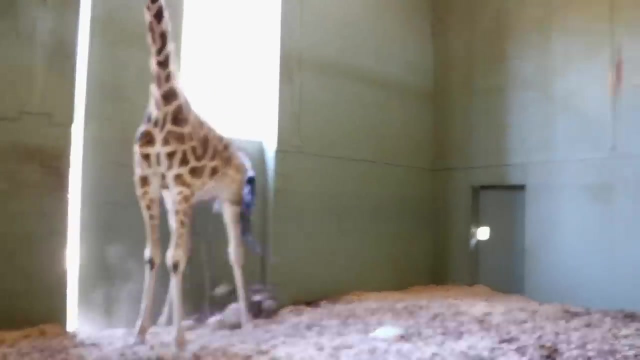 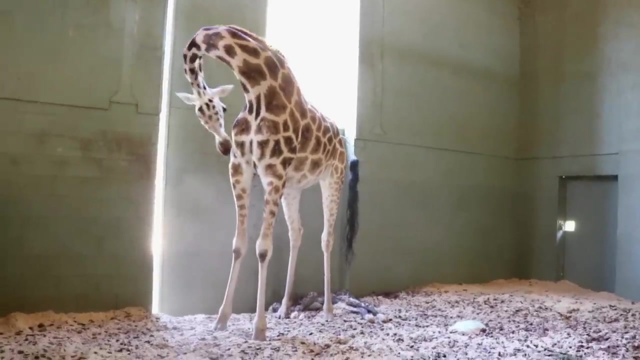 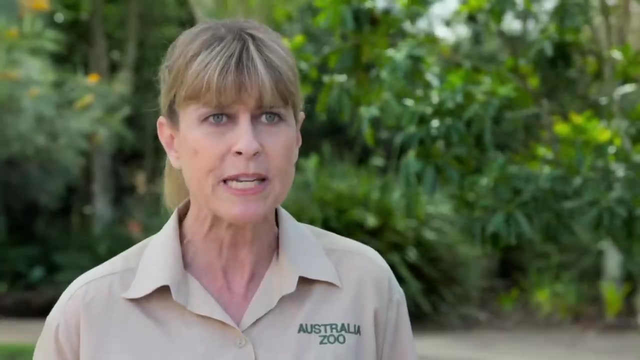 the way the calf falls out, But certainly a little bit of an anxious moment. Oh, cat, cat, it's happening. Oh my god, not at the right angle. There you go, It's all right. Dropping about seven feet to the ground for a new baby animal is a little bit terrifying. 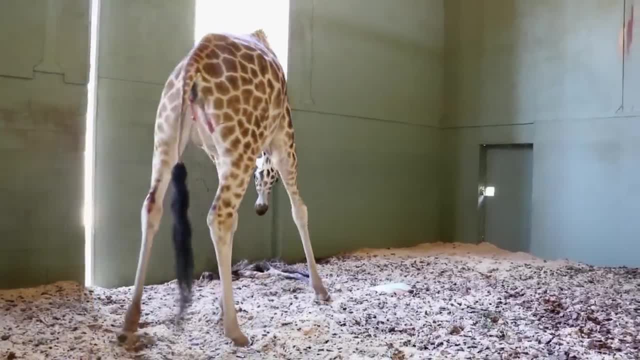 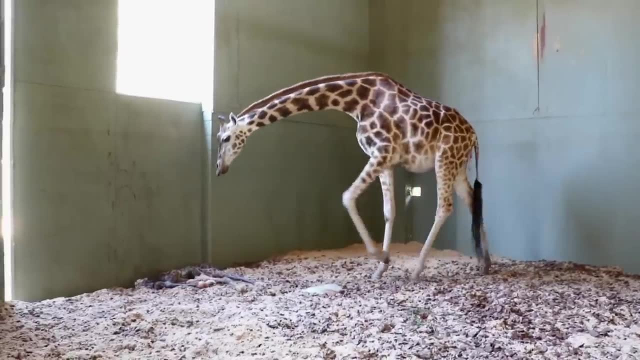 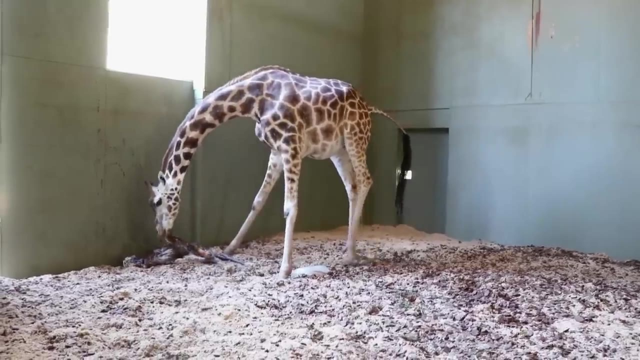 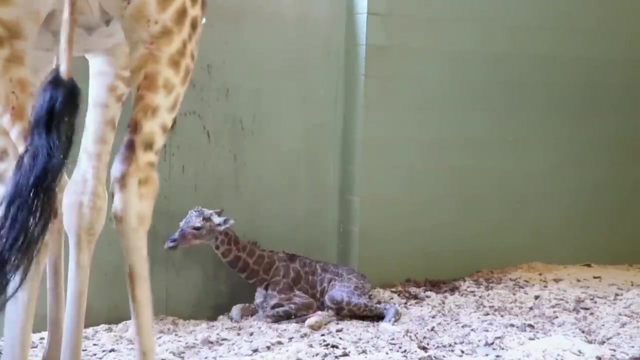 And then making sure that the baby's breathing okay and there's no problems or complications. Every step of the way you're kind of a little bit nervous. Good girl, Wow. I am so, so happy. The entire zoo has a buzz floating around because this beautiful giraffe has officially been born. 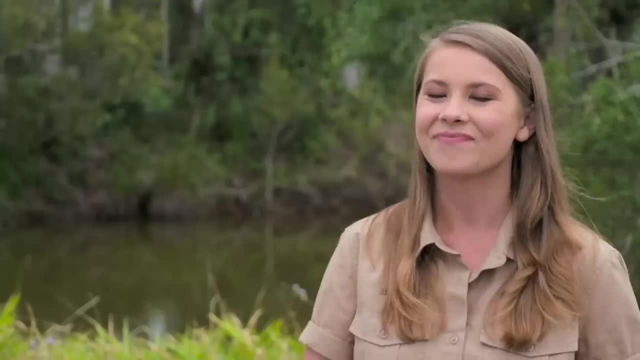 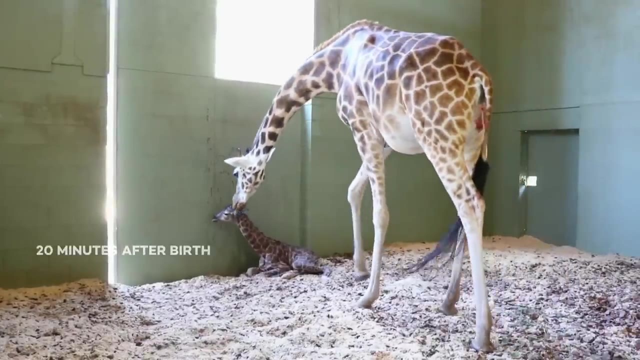 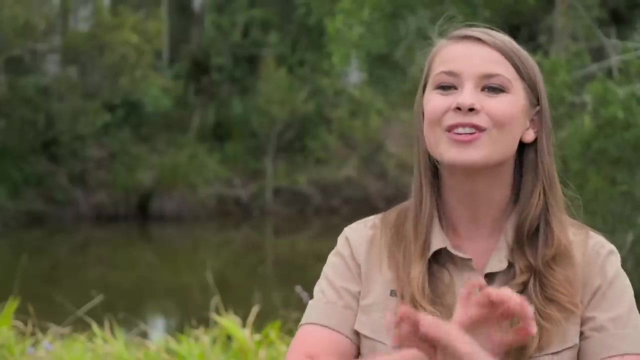 We have been waiting 15 months for this moment, So we're pretty excited. Our little giraffe is doing really well and she's so gorgeous. Oh my goodness, I am so, so excited, I'm so happy and we are just absolutely thrilled. 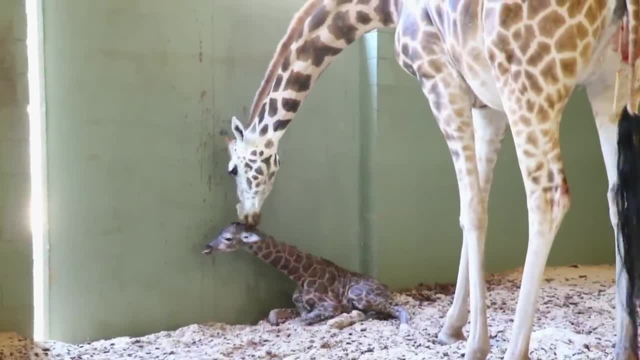 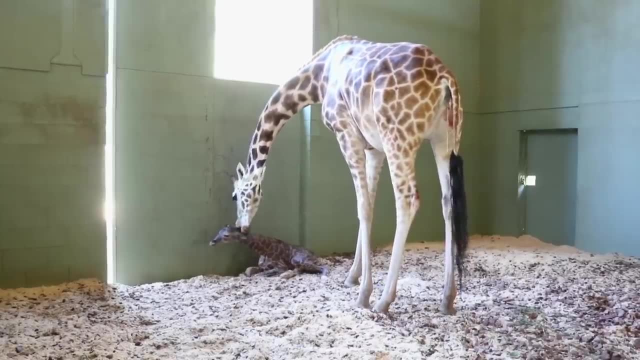 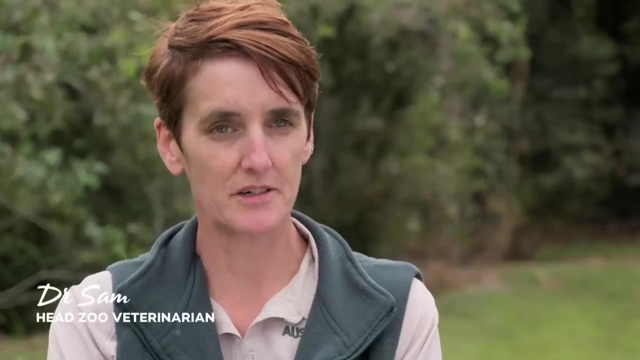 My whole family is excited. Rosie's had her baby and everything went perfectly. We're just really looking for strength and alertness and then ability to get up off the ground and start cycling. Those are the most important things, and we try and do that without. 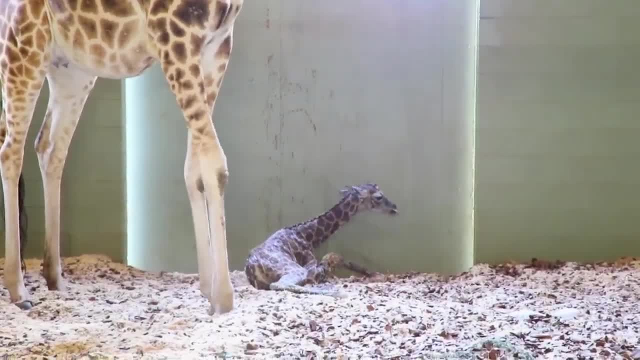 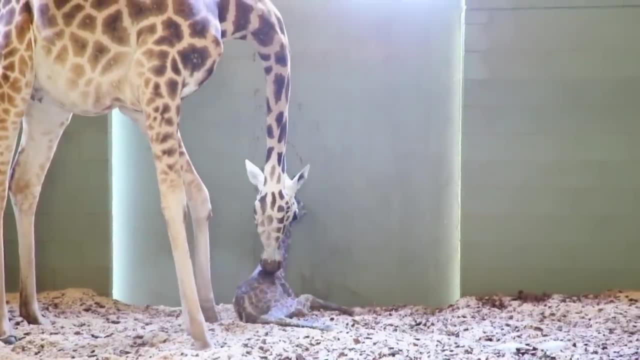 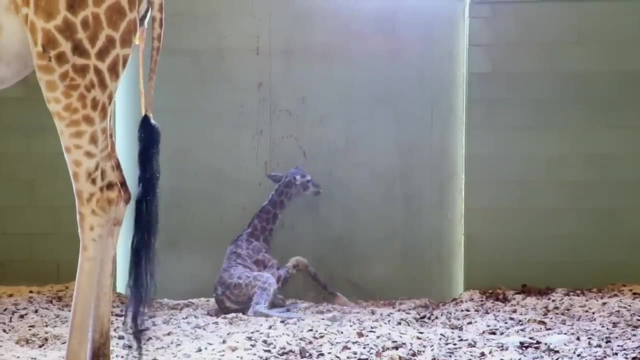 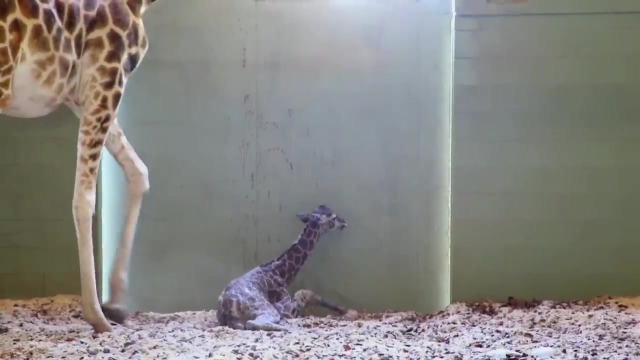 interference with mum and calf. We really want them to bond quickly, So minimal human interference. She's trying to stand up. The first hour of a giraffe's life is extremely important. In the wild there's a lot of animals that might think a baby giraffe is quite delicious. 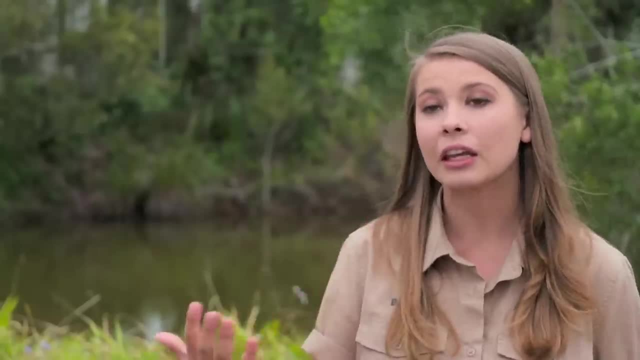 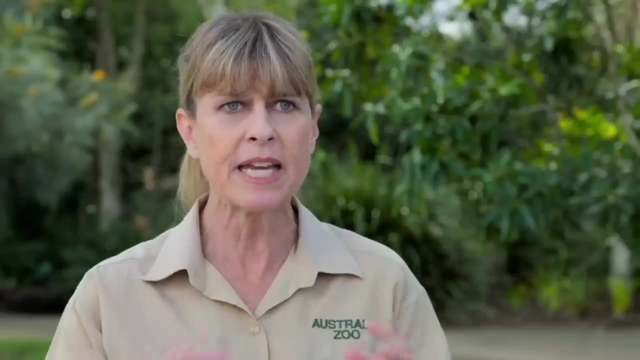 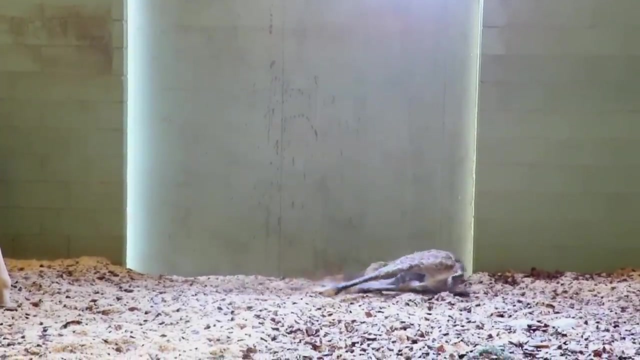 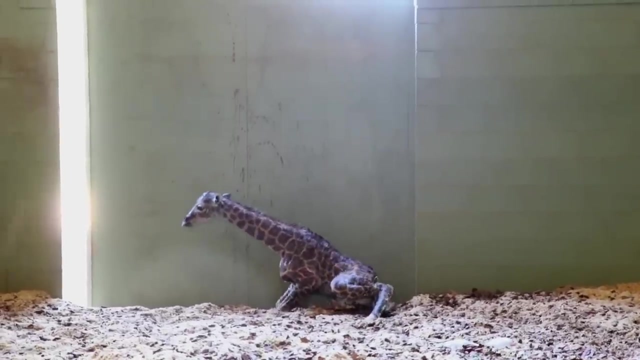 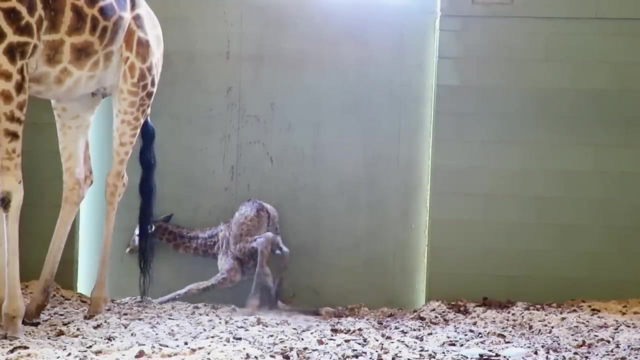 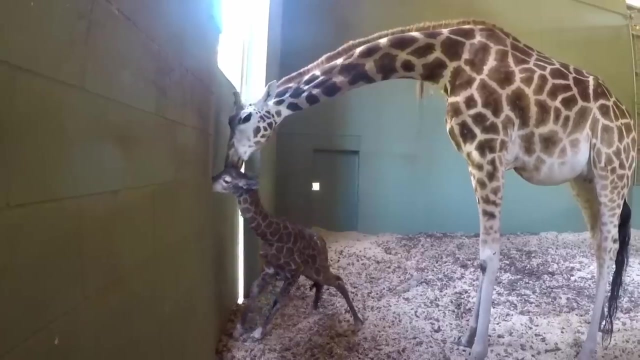 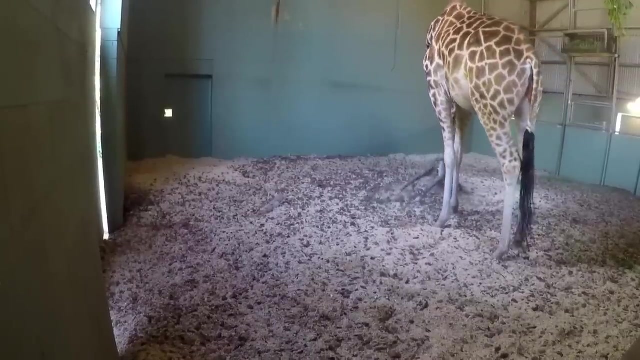 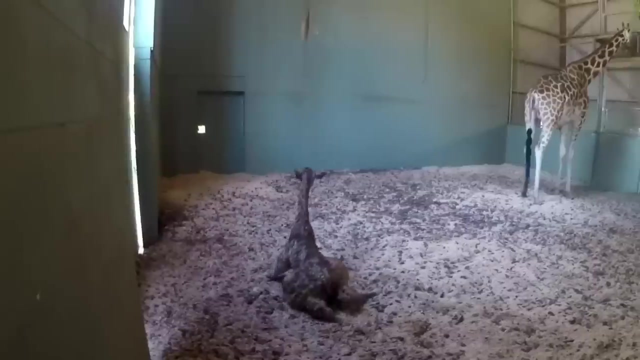 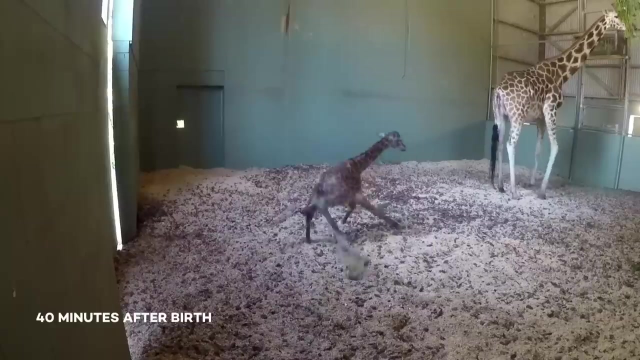 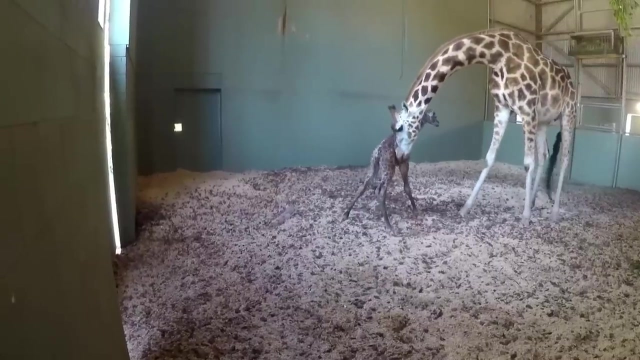 So little giraffes need to learn to stand and stick really close by their mothers. You do feel a little bit helpless. helpless because they kind of fall and crumple to the ground. Oh baby, So hot. Good girl, You want to help your baby. 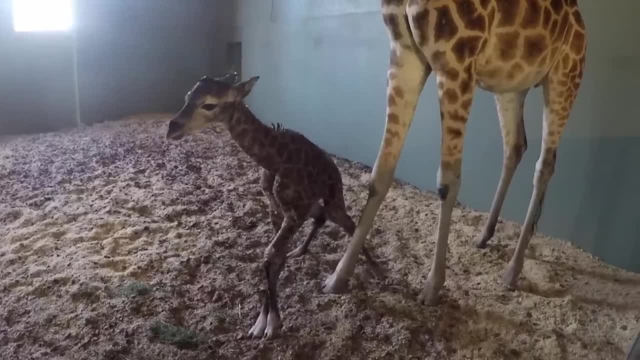 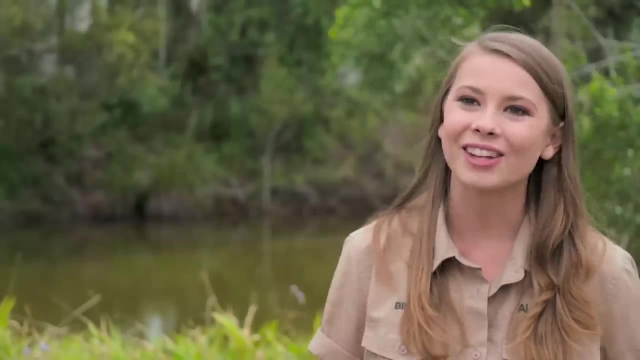 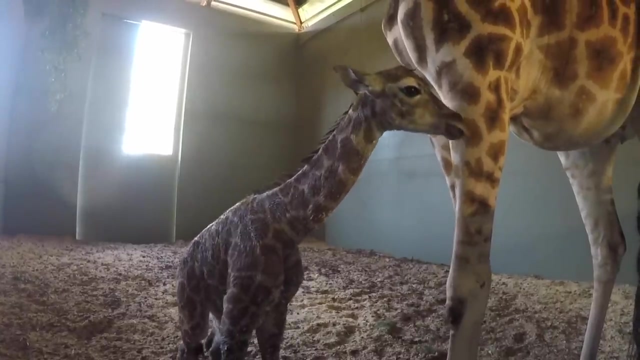 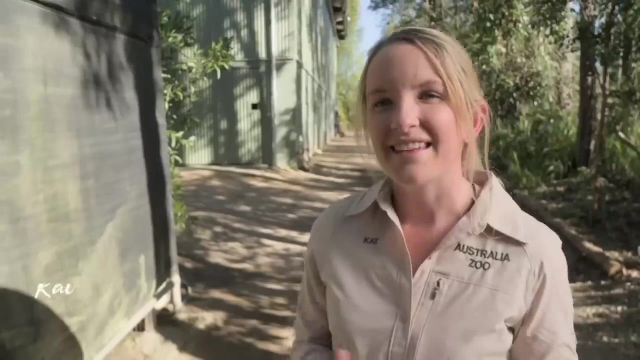 Good girl, Rosie. Rosie is such a great mother. From her first calf she has always been very attentive. She's been very dedicated in making sure her little one is strong enough to stand and stays close by her side. The next big milestone that we're waiting for. 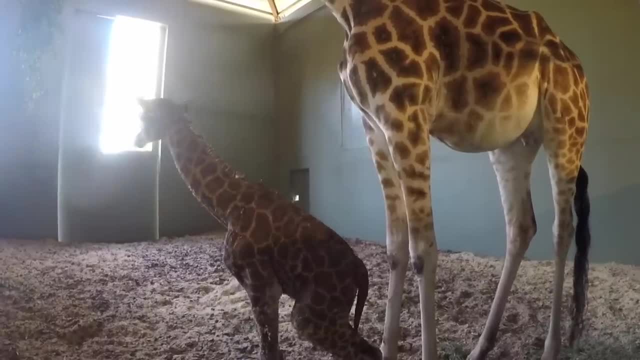 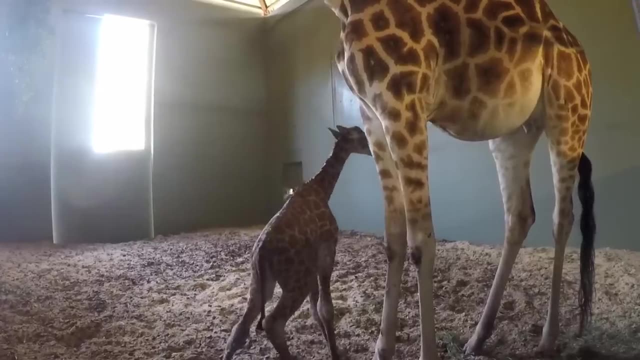 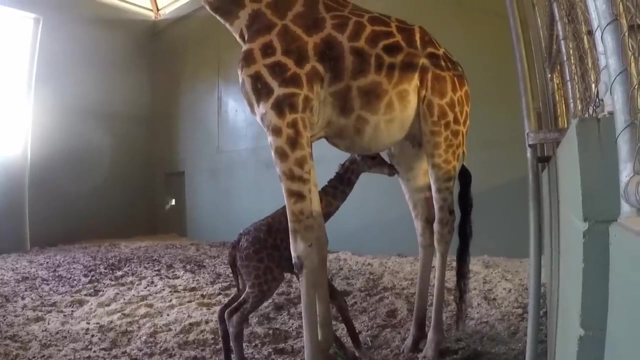 is making sure that calf actually suckles, because obviously it's a big deal That is essential for a growing calf. You're going so well, Good kid This way. Hey, hey, hey, Listen up there. So in the next couple of minutes, 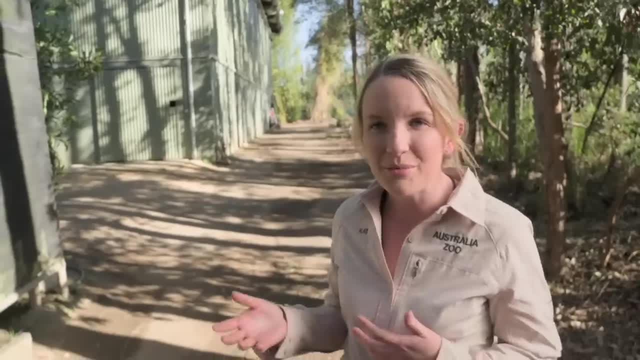 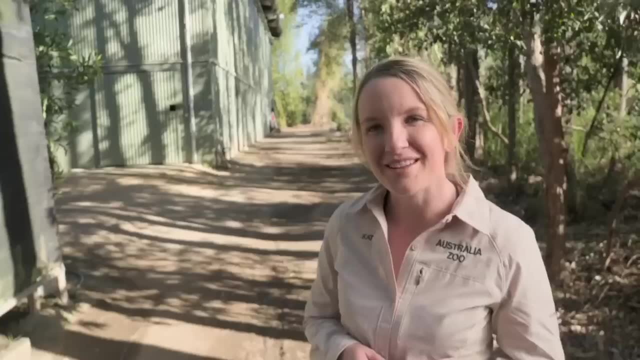 we're going to be able to see if little one has a drink. Mum's actually pushing her in the right direction as well, But she's quite wobbly on her legs, so we're not going to be able to see her. She's a bit more relaxed. 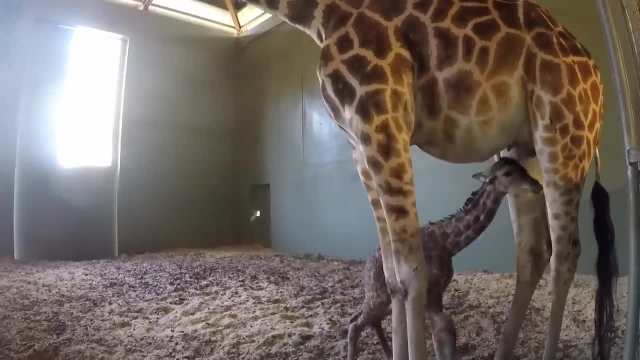 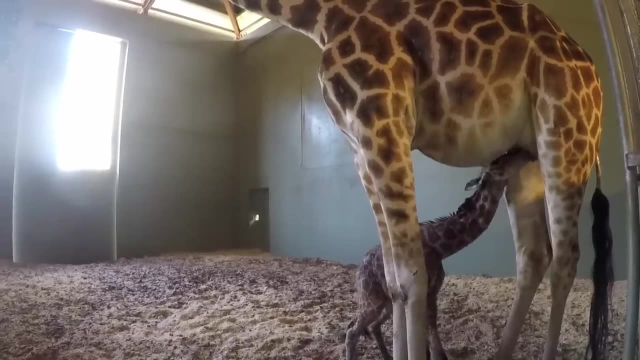 Alright, We've actually been able to see four little teats, so we know that she's a little girl. We're getting a little closer now. It's good. it's good, That's gonna do it. Okay, that's good.